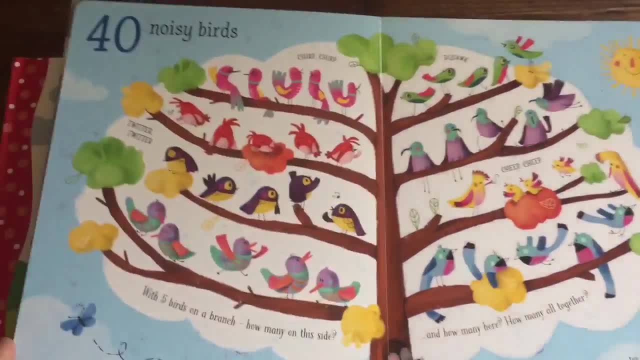 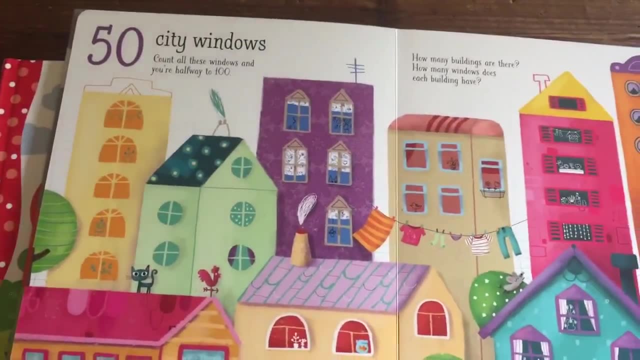 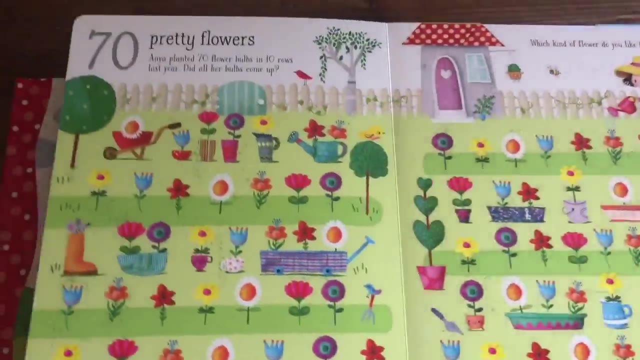 over and over again and you're not worried about pages ripping. I love that illustration, Isn't that darling? It's great to practice counting and working your way up to, or your child working his or her way up to counting to 100, and learning to count into groups. I love this page. I think. 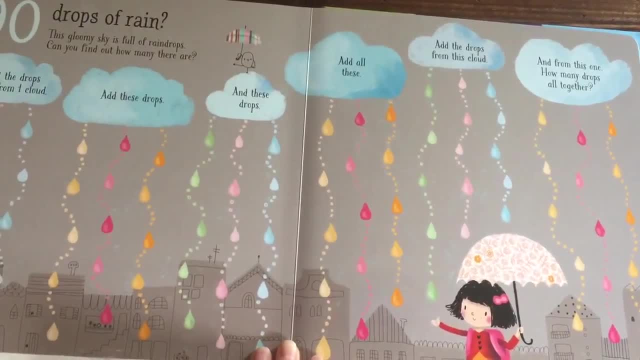 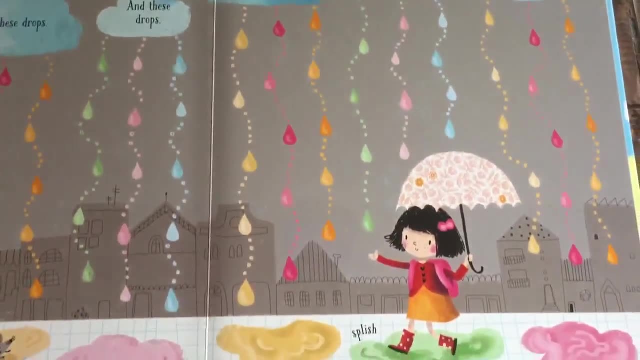 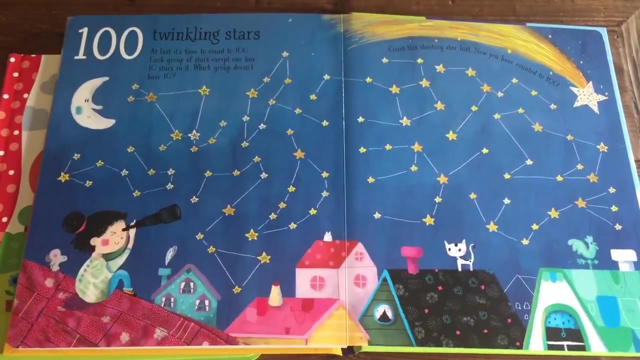 that's pretty awesome. See how on the clouds it says add these drops. So you're actually counting into little groups, You're grouping your numbers as you're getting up into the higher numbers and look at 100.. It's the constellations, the stars in the sky. I just think it's fabulous. 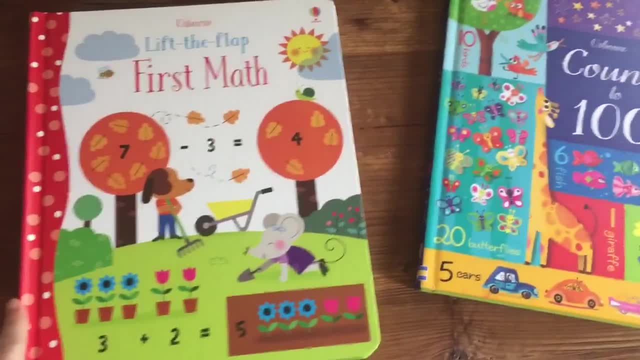 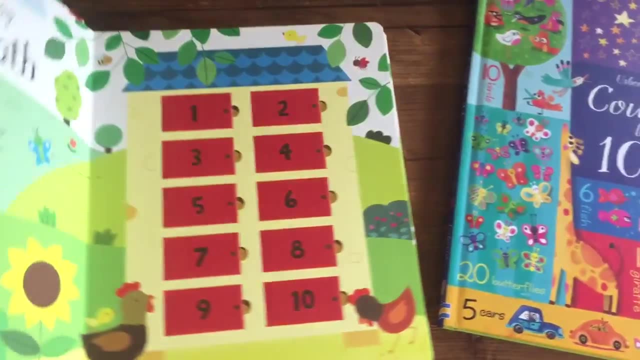 Then last year for kindergarten math, this was my daughter's. she called it her math book. Of course, it wasn't the only thing we did for math, but it was such a great supplement. She still loves going through it and now we can work through it so easily because she knows it all. 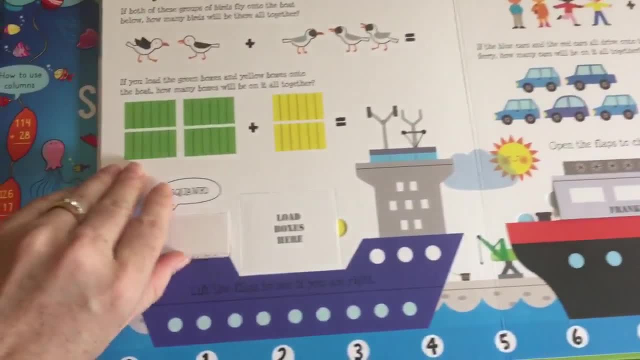 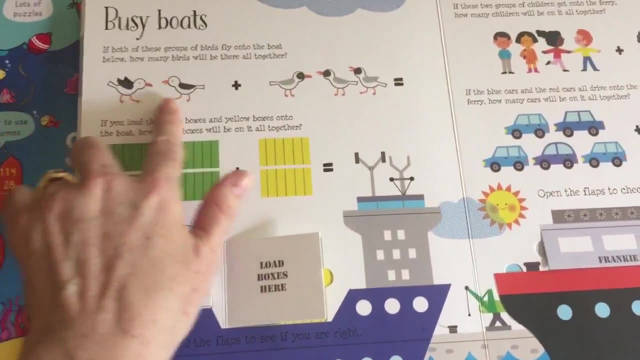 She's learned it all. It's simple edition and these are the lift-the-flap books that we adore from Usborne. You solve a little problem up on top and then you lift the flap and then you go ahead and bring your book home. It's a simple, easy way to start your day. I'll share the link in: 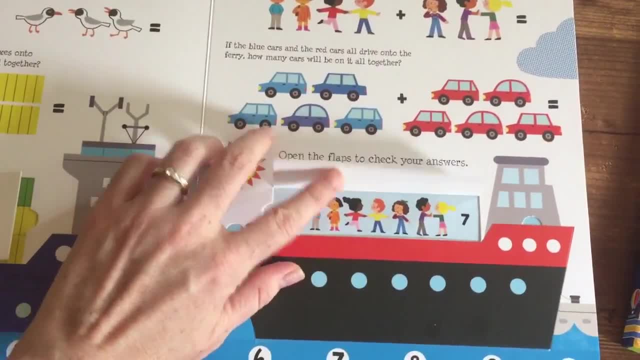 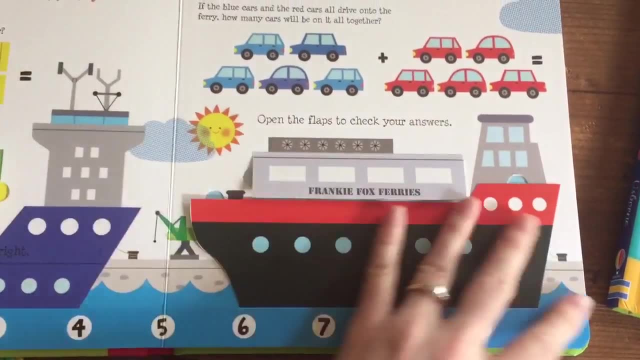 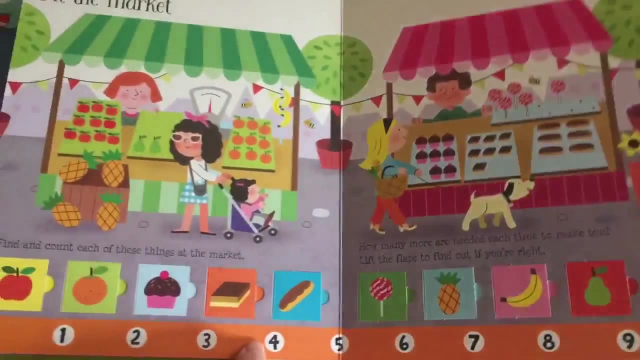 Lift the flap to check your answer and see if it's correct. She has so enjoyed this. Oops, download. there we go. There's all the cars, I think. our favorite page. we love the flowers. Our favorite page is this one: 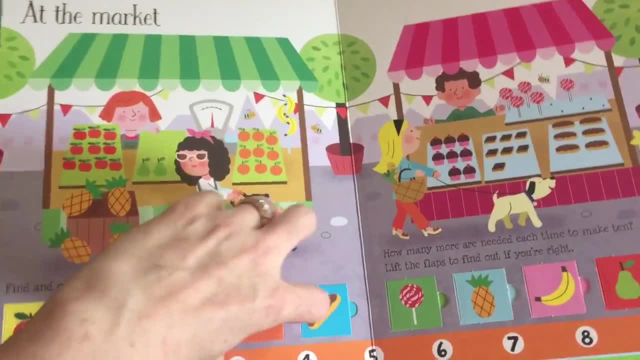 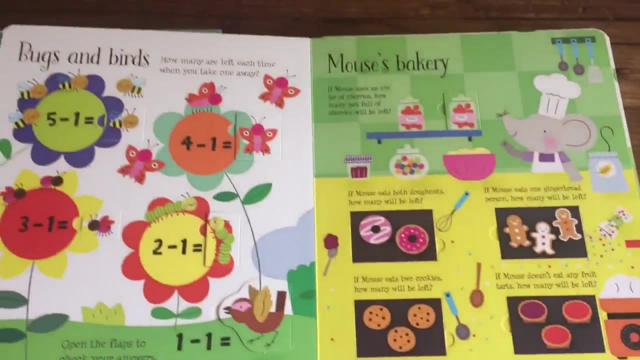 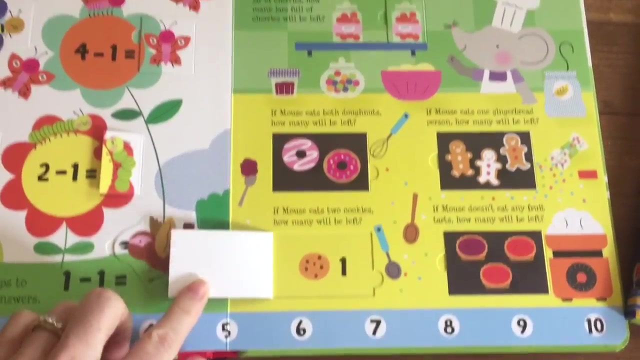 the farmer's market isn't that cute. So this was such a wonderful fun. engaging. simple activity book for her this year as we learned, simple addition And then we're going to move up to this book this year. Now I will say I am actually going to give this book. 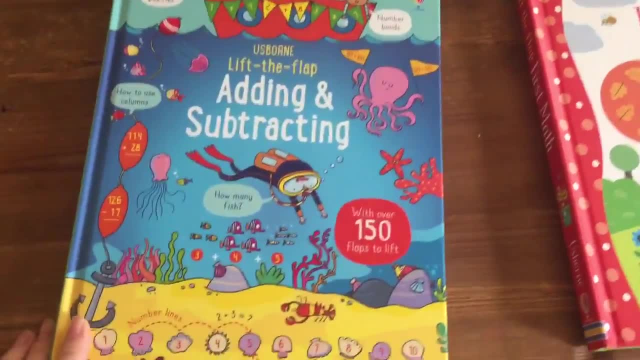 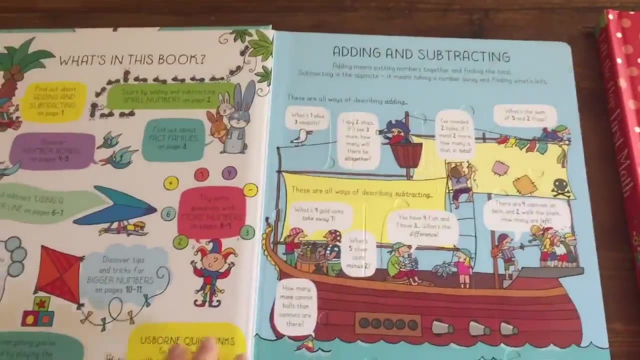 to my fourth grader and have her do the same thing. So I'm going to give this book to my fourth grader and have her do the same thing. So I'm going to give this book to my fourth grader and have her do the same thing. 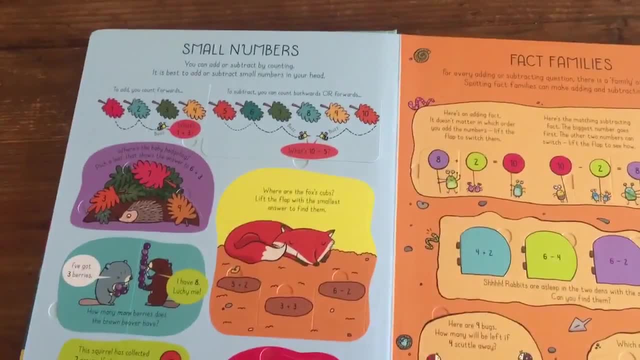 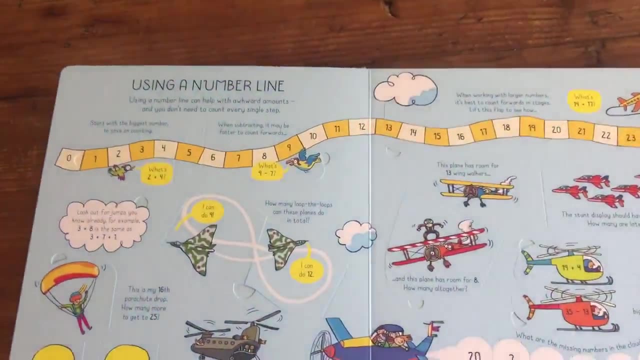 And then we're going to do some reviewing with it because it's actually quite advanced at the end. It starts simple small numbers and fact families and it goes into number bonds and using a number line You can see that the flaps are not popped up yet. 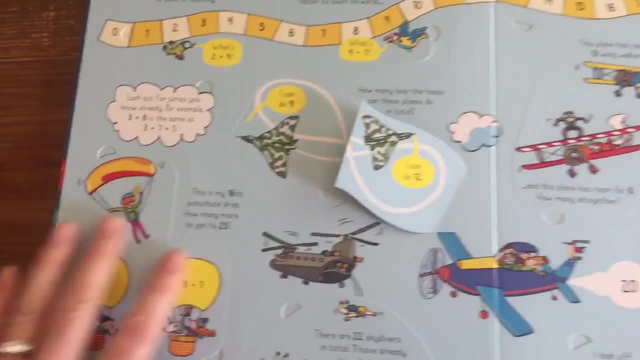 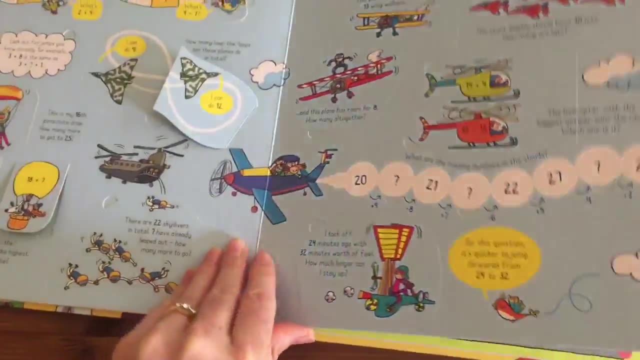 because we haven't actually used it yet. I'm so excited to use it And I can see that this is going to be a wonderful resource and it's going to take a long time to work through. And it's going to take a long time to work through. 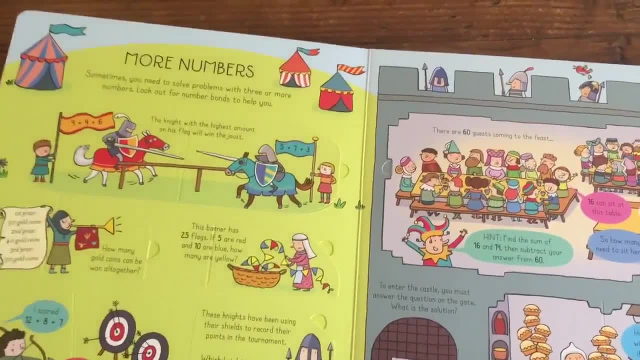 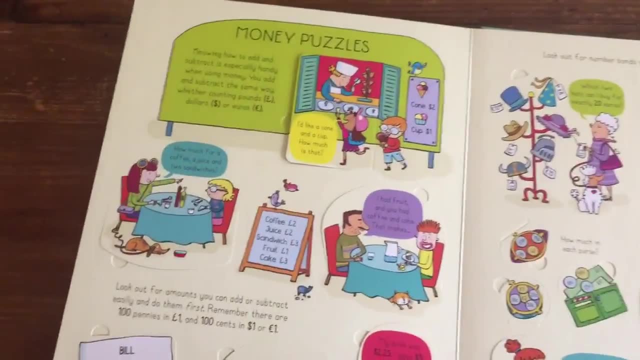 Which is good. it's not something that's just gonna happen in one sitting and then look at how advanced it gets here at the end. let's see, it has money puzzles. this one's popped up. I think my daughter's actually looked at this one already a little bit. 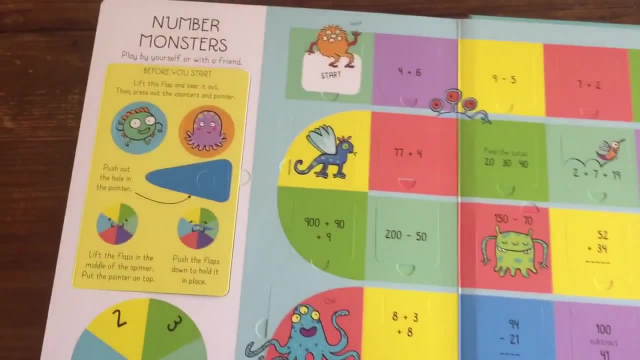 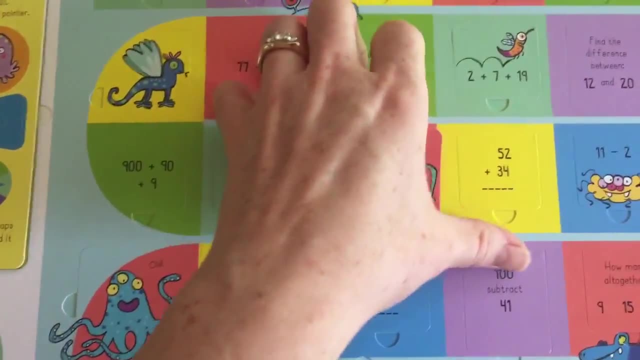 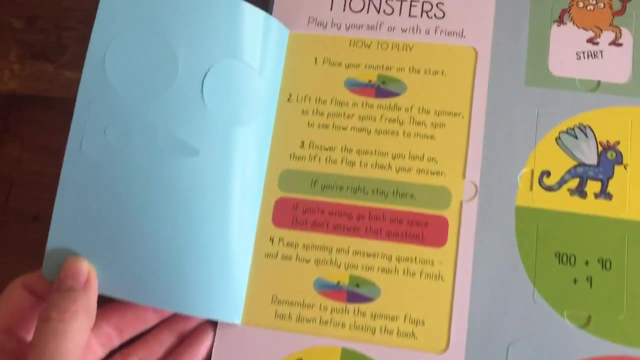 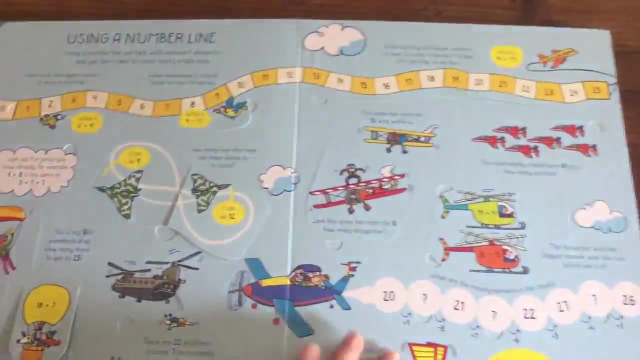 and then the number monster here at the end. thank you, my youngest likes monsters, so I think she'll enjoy that. how to play gives little instructions. what I'm planning on doing actually is having my older daughter work through this with my youngest daughter. of course, I'll do it with her as well, but I think it's just 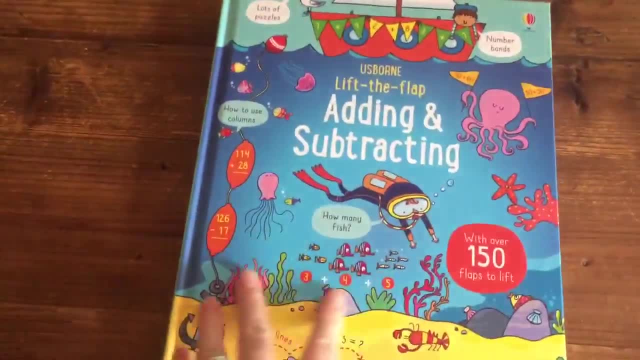 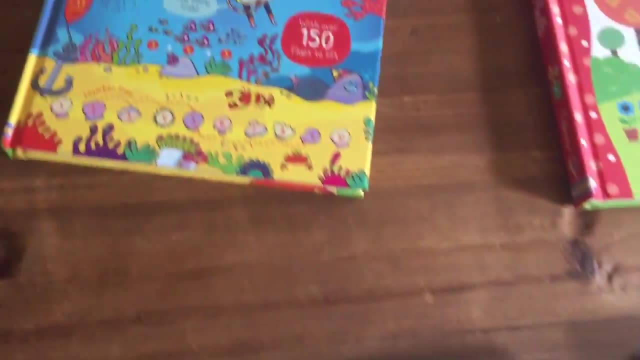 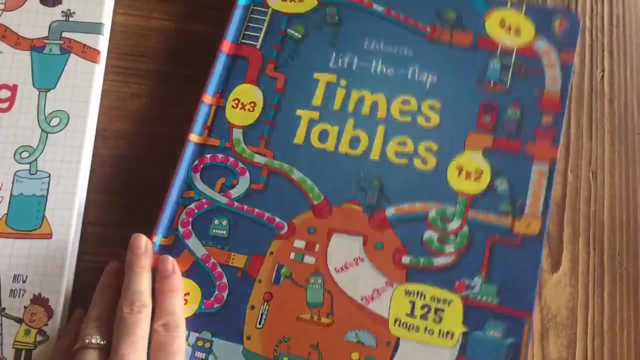 gonna be a fun activity book to support us as she learns higher levels of adding and subtracting. then for my oldest daughter, my fourth grader last year, I, I, I, I, I. we worked on the times tables and she had to memorize her times tables and man. 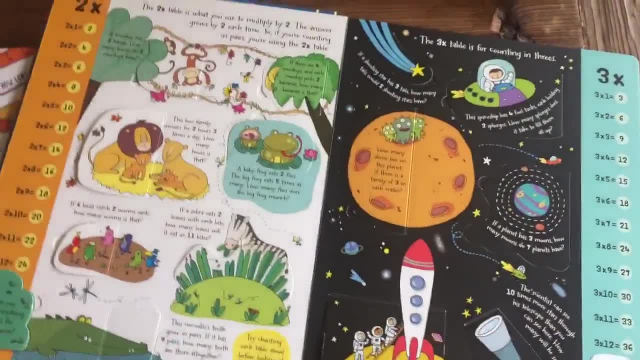 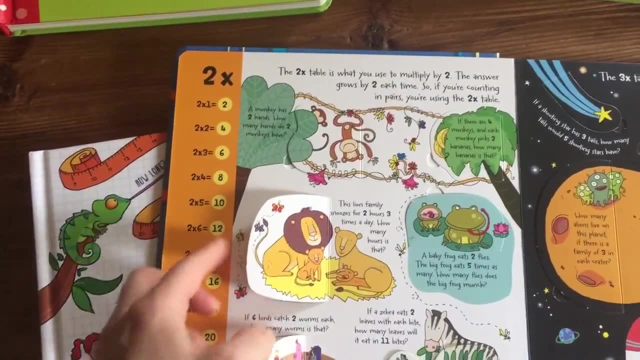 oh man, this book was a lifesaver. I would give her this book and I would say: okay, work on your twos. and you could see how these are all flapped up because she has been working on them and or she did work on them, I should say, and she would go. 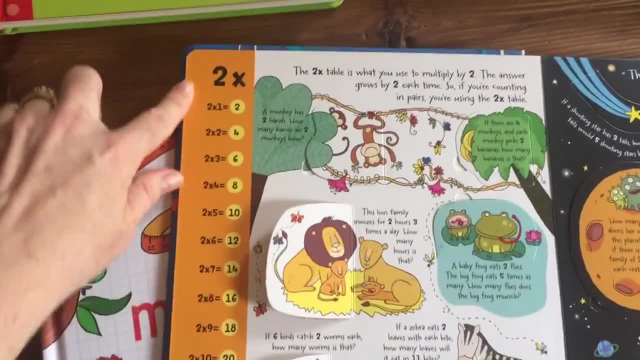 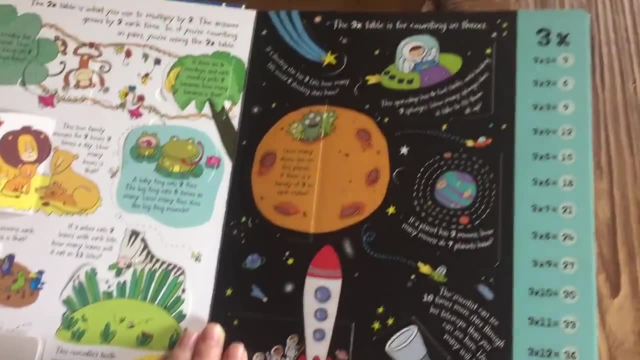 through all of the flaps. she would go through all of the the times tables for the twos and she would memorize them, and then the next day I would say, oh my gosh, okay, let's work on your threes, and so on, and went on for a while, all the way up to. 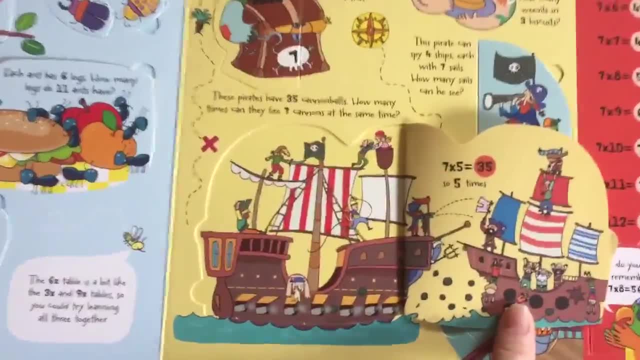 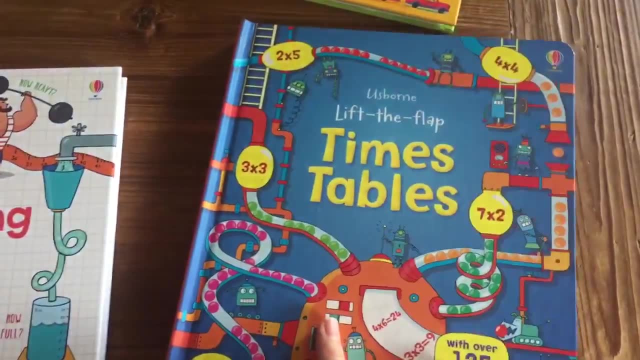 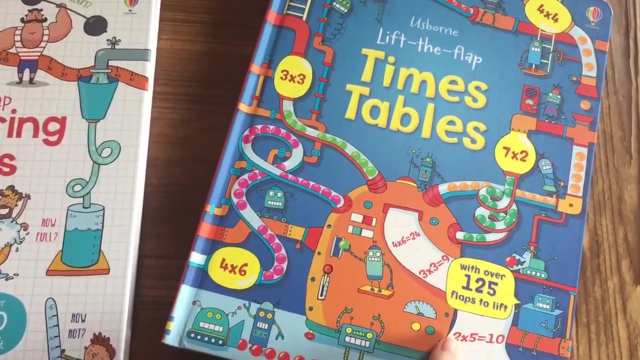 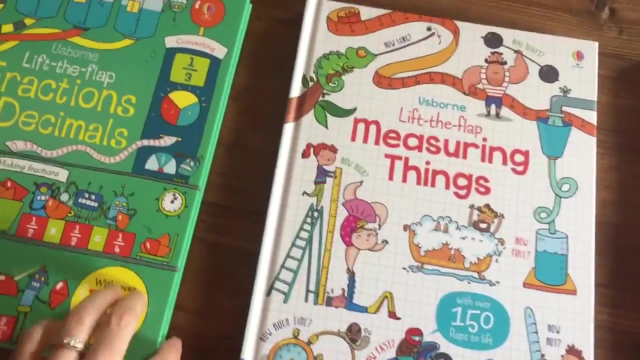 twelve with cute engaging illustrations and examples all along the way, and she used this and the wrap-up that also comes from us forum and it was just such a wonderful resource for her 125 flaps to lift in this book. so I have added the fractions and decimals and the measuring things books. 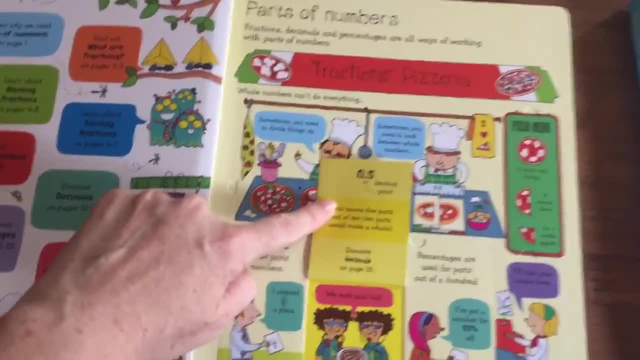 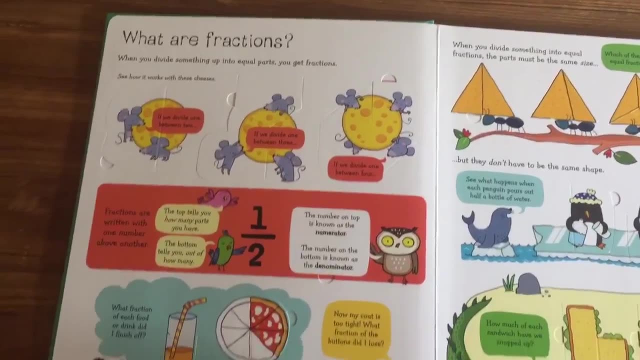 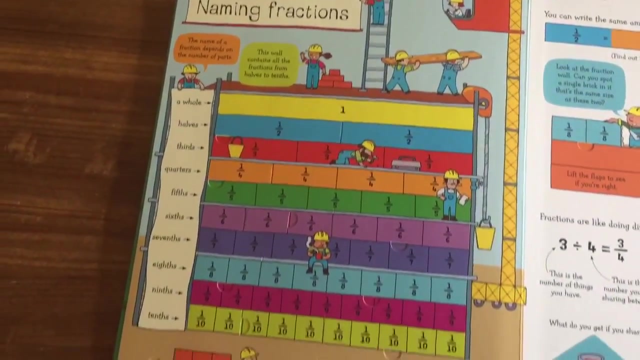 for her for this year and you could see we haven't really lifted them yet, but I think these- if there anything as bright as the other math books have been. I am so looking forward to using this with these with her. usually with something like this, we have to go through it together. at the beginning, we sit. 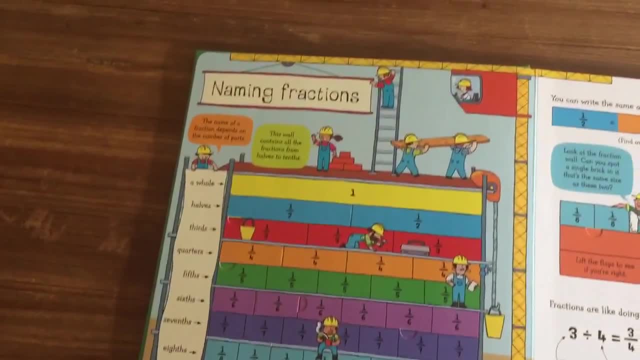 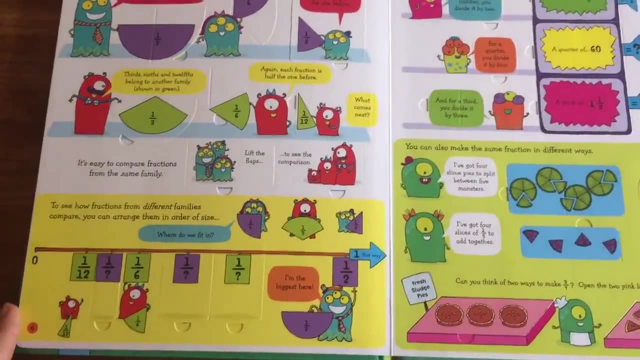 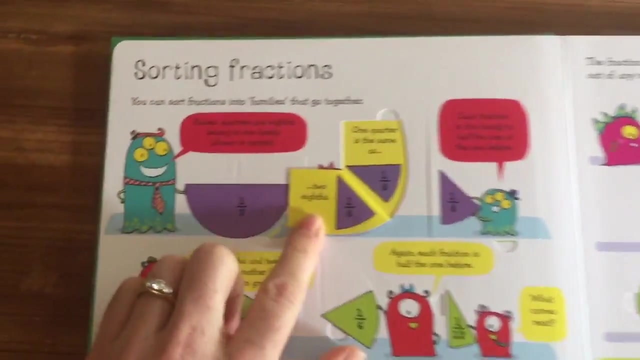 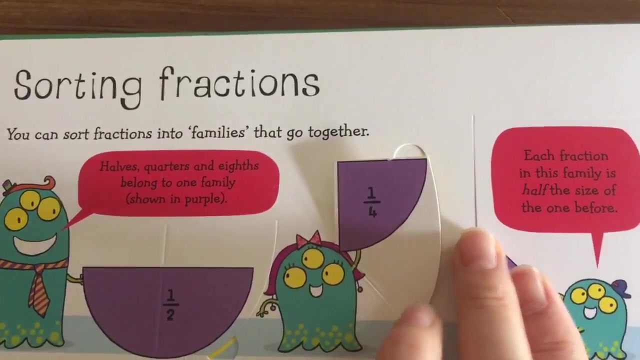 together and just walk through one page or maybe even half of a page. that's the great thing is, this book is gonna actually last a while. it's not something she's just going to flyeland in one sitting sorting fractions, one quarter, two eighths. one quarter is the 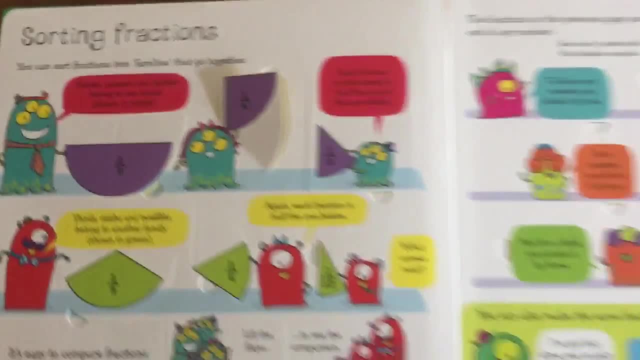 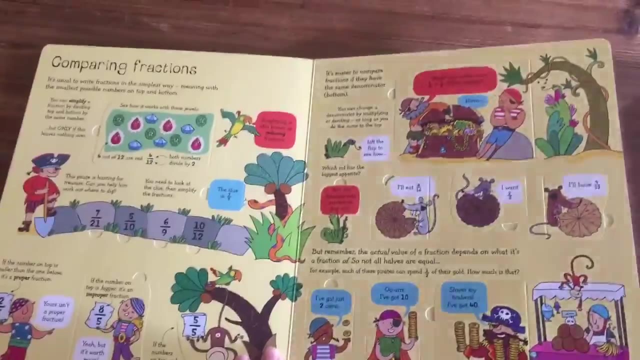 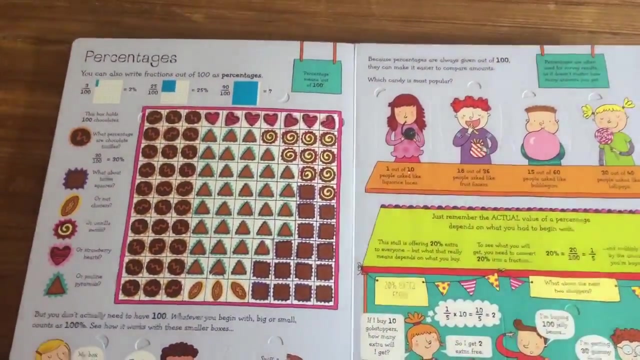 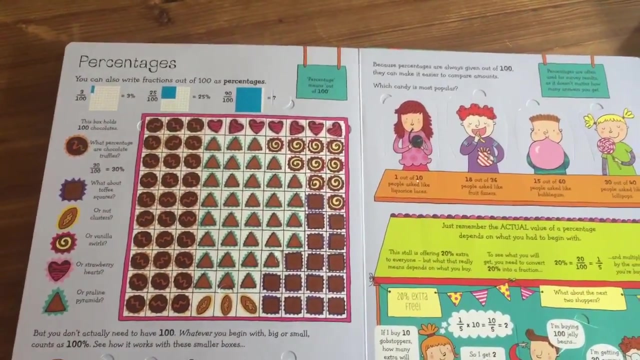 same as two eighths. this is also a wonderful thing that can be worked through with a math tutor. if your student has a tutor, what a fun thing to do with a tutor to say, okay during your tutoring time. today, work through one spread of this fun math book that's working on decimals and fractions and 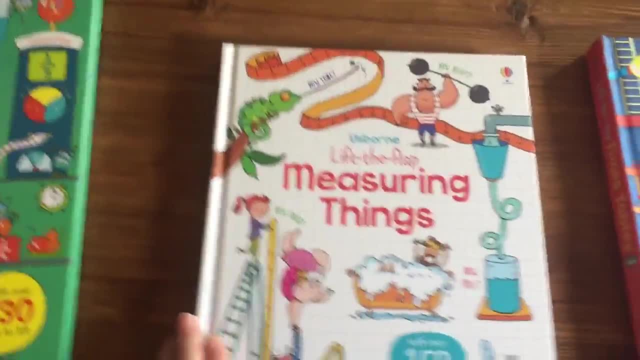 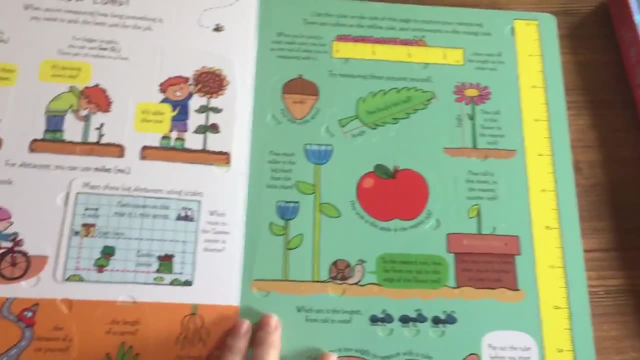 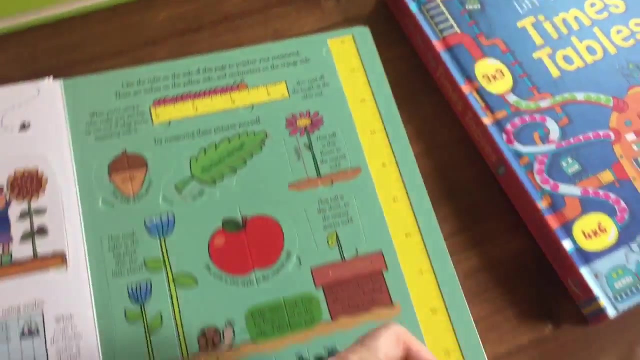 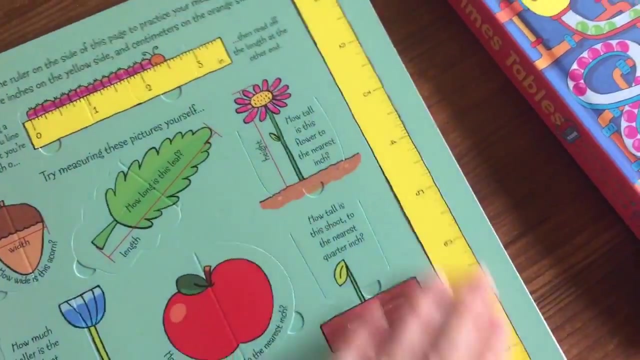 percentages. same thing with the measuring things. now this one I'm planning on, after working through a page together, then actually going and getting. now I know this ruler actually pops out, isn't that cool, and it has the inches and the centimeters on the back and then you can. 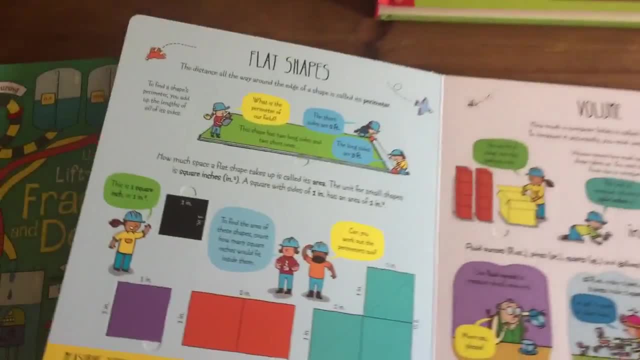 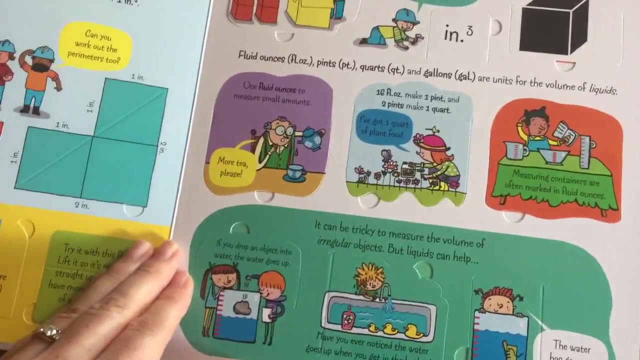 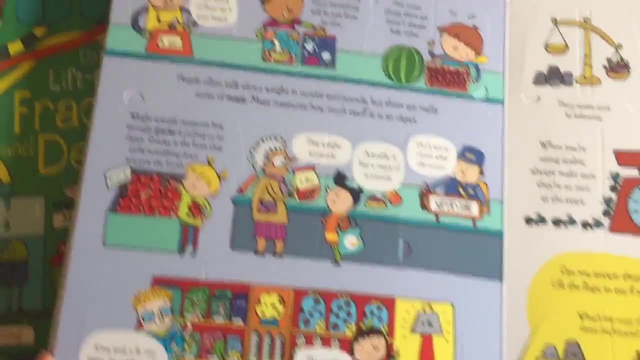 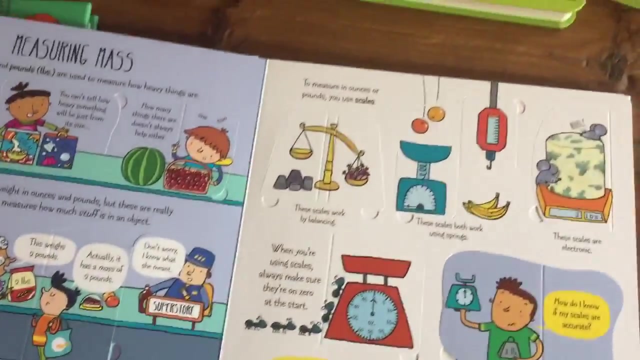 use it. but I'm planning on then doing examples of it in our home, like, for example, whenever we do volume, getting different kind of doing the book and then illustrating this with actual things that we have around the house. I have a scale. I'm planning on pulling out the scale whenever we do this page, so I 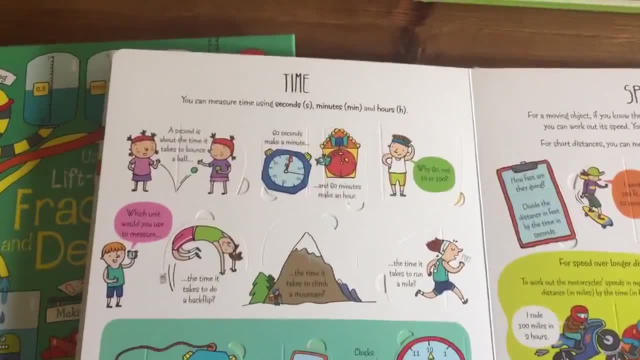 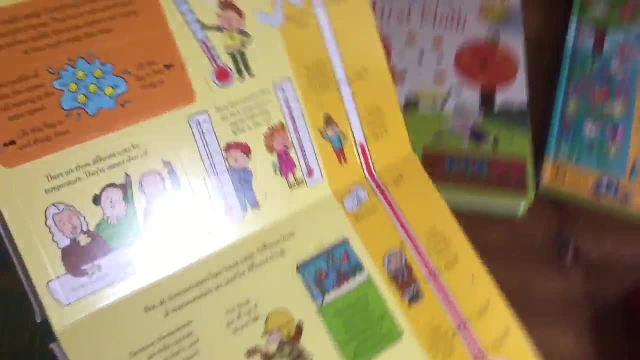 think it'll be really fun for us to do the page together and then go play with some things that are actually what is illustrated in the book. so, as you can see, these are some office叙迫. WHAT ARE THESE USE BOOKS GOING TO GIVE US ON THE C? zap?